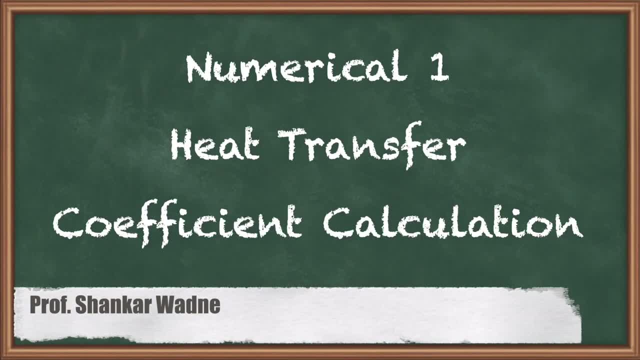 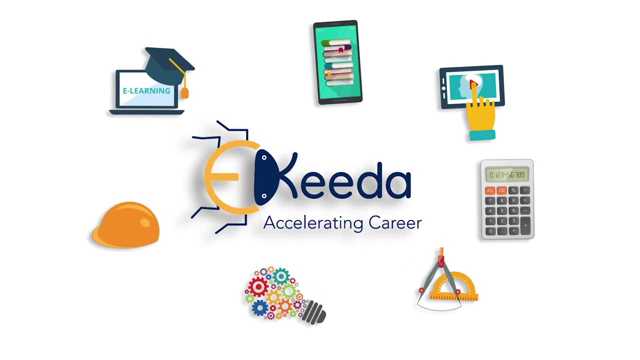 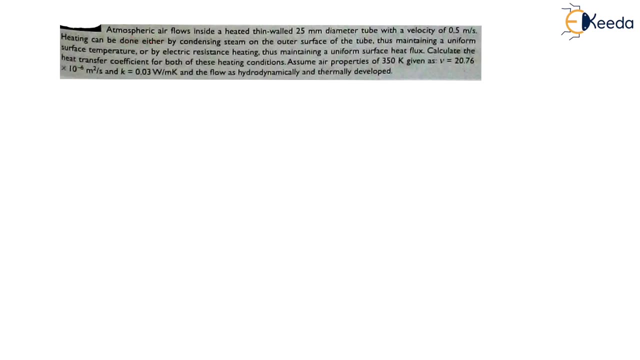 Hello, my dear students, In this lecture we are going to see one numerical on convection to find convective heat transfer coefficient, EIJ. So let us understand the question. The question is: atmospheric air flows inside a heated, thin walled 25 mm diameter tube. 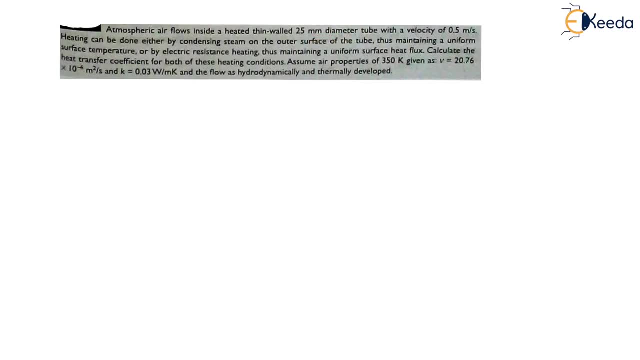 Now, here air is flowing through a tube or diameter tube means it is a cylinder. Let us say there is a cylinder like this. Let us say this is a cylinder, Through this cylinder the air is flowing. Through this cylinder the air is flowing. Therefore, inside I can say there will be a air. 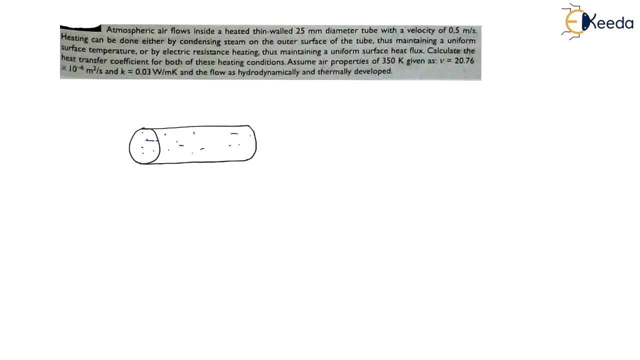 Inside there will be a air through this tube which is flowing. Let us say the diameter of tube is given. Here the diameter will be D and length will be L. Length will be L and diameter will be D. Here diameter is given to the tube. 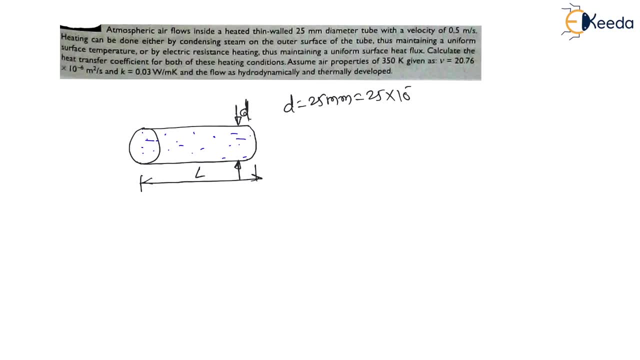 25 mm, 25 into 10 to the power minus 3 meter. Then air is flowing through this With a velocity of 0.5 meter per second. This air is flowing with a velocity of Now the velocity of flow is given 0.5 meter per second. 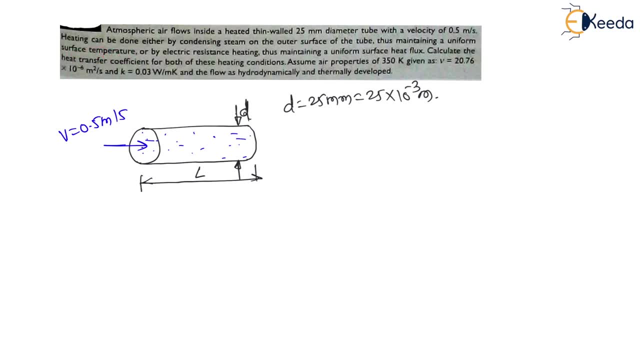 Then heating can be done either by condensing steam on the outer surface of the tube, Thus maintaining a uniform surface temperature. Now, my dear students, for this wall, the heating can be done by condensing steam. Now, here to outside this tube, there is a steam. 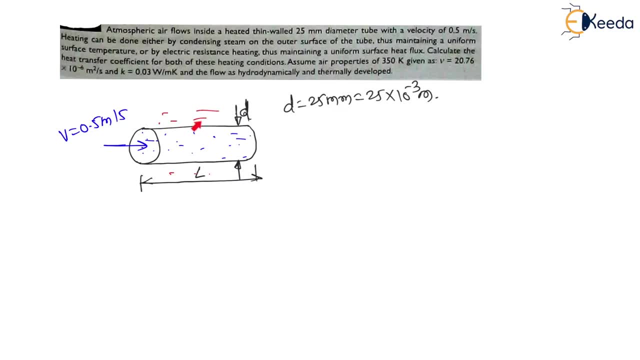 Here outside this tube there is a steam And this steam may get condensed to get this tube heated And thus they have mentioned thus maintaining the uniform surface temperature Means the first type of heating is uniform surface temperature, Uniform surface temperature, That is, constant surface temperature. 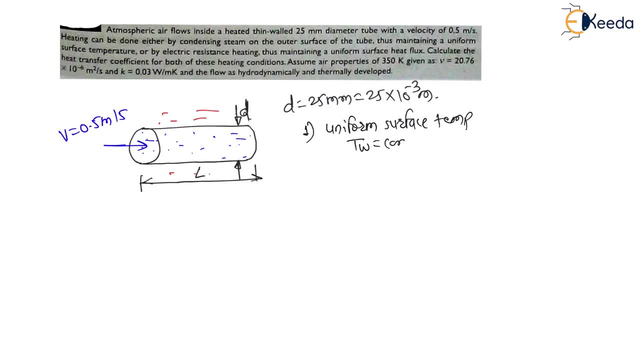 That is wall temperature. Wall temperature will be constant. This is the first type of heating. Let us say the tube wall temperature is T wall. Tube wall temperature is T wall, That which is constant. This is the first type of heating. Now, second type of heating is: or by electric resistance heating. 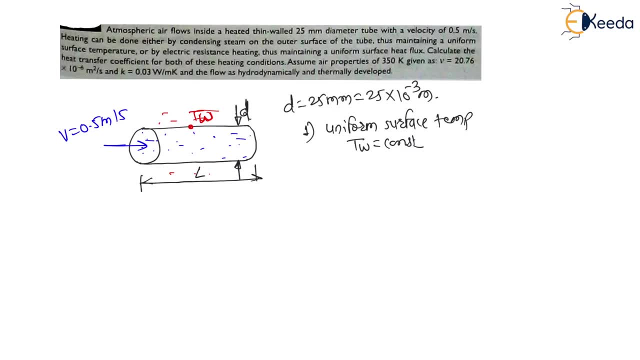 Thus maintaining a uniform surface heat flux. Now, second type of heating is around this tube. The coils are wound And because of this coil they are heating this tube such that it maintains a uniform surface heat flux Means. second type of heating is for uniform heat flux. 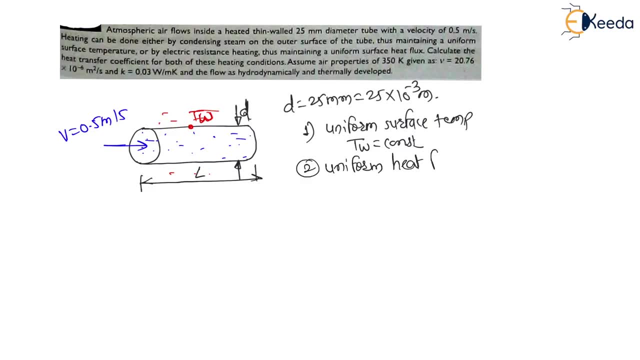 Uniform heat flux, Which is the thing. But here heat flux Q will be constant, Which is Watt per meter square Is constant. This heat flux will be constant. These are the two different types of heating. Right Now Calculate the heat transfer coefficient for both these cases. 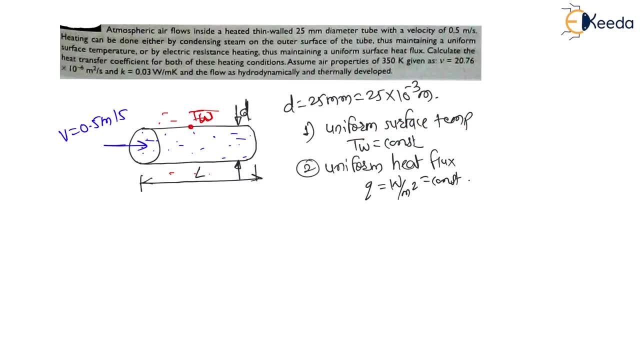 Now here for uniform surface temperature as well as for uniform heat flux. Calculate convective heat transfer coefficient E- h. We have to calculate E. h Will be question mark. E, h will be question mark Right For both these heating conditions. Assume air properties of 350 Kelvin, given as 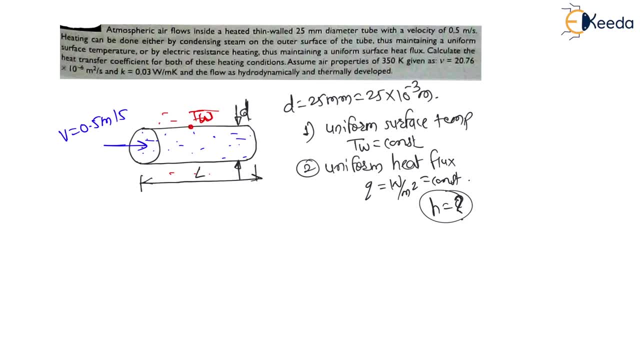 Now the air temperature is 350 Kelvin, Means surrounding fluid temperature T infinity is given 350 Kelvin And the air properties are given. Here kinematic viscosity Meter square per second is nothing but unit of kinematic viscosity, Right. So here kinematic viscosity is given. 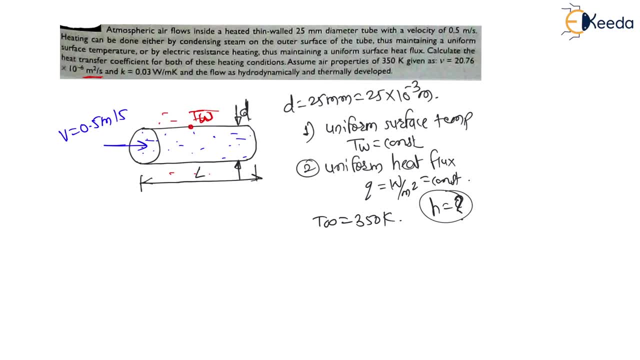 20. Here it is a Kinematic viscosity nu is equal to 20.76 into 10, to the power minus 6 meter square per second, Which is nothing but dynamic viscosity, They have a mass density Right. Then thermal conductivity is given. 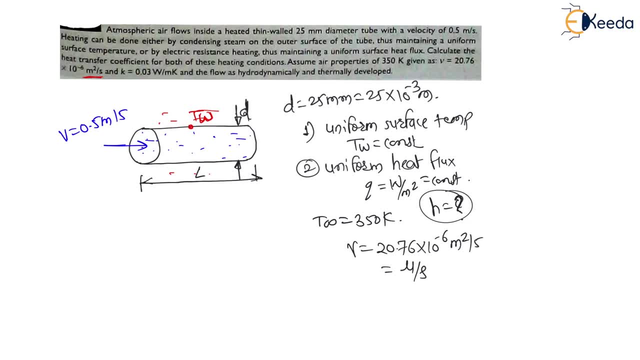 K is equal to 0.03 Watt per meter Kelvin. Therefore, thermal conductivity is given. Therefore, thermal conductivity of air is given 0.03 Watt per meter Kelvin Right And the flow as hydrodynamically and thermally developed. 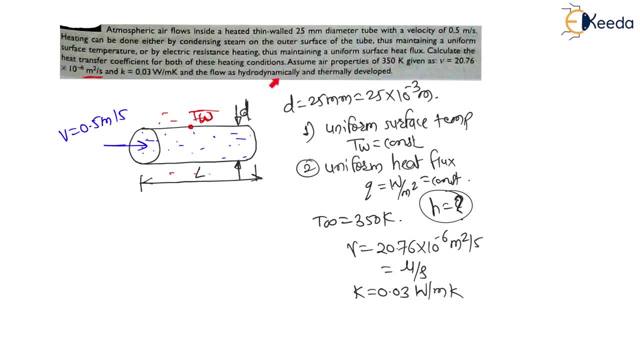 Now, here, the flow is hydrodynamically as well as thermally developed. Right Now, my dear students, first of all, for such type of flow, let us calculate Reynolds number. Now, Reynolds number is nothing. but for flow through pipe, the Reynolds number is rho Vd. 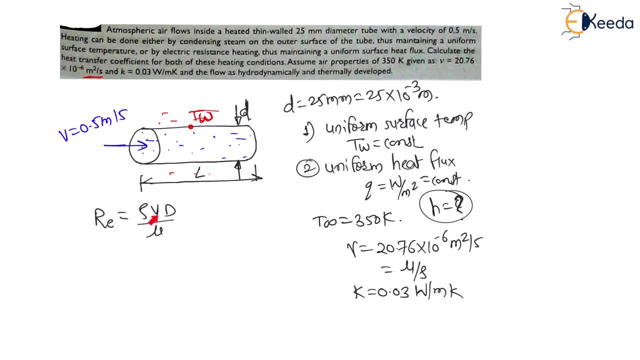 upon mu, Where rho is density, V is velocity, D is diameter of pipe and mu is here dynamic viscosity. Therefore it will become Vd divided by mu by rho, because diameter of pipe is, we have written small d, Mu by rho. This mu by rho is nothing but kinematic viscosity. 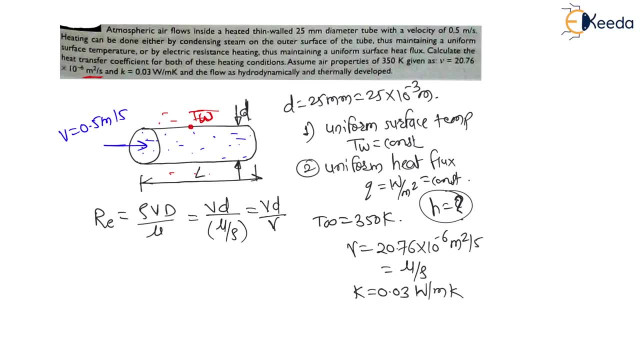 Therefore it will become Vd divided by kinematic viscosity. Therefore this Reynolds number for this pipe will be equal to velocity, is 0.5.. It is given diameter is given 25 into 10 to the power minus 3.. into 10 to the power minus 3. into 25, into 10 to the power minus 3, you have a kinematic viscosity. 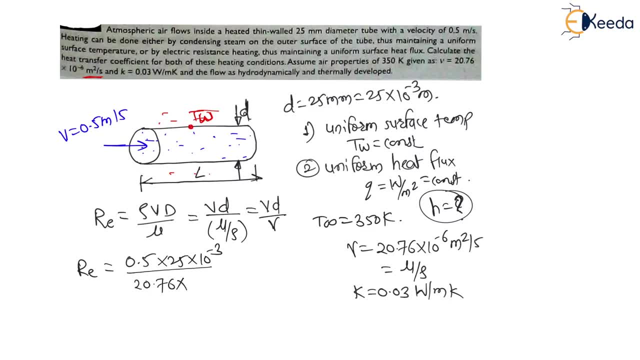 kinematic viscosity is given 20.67 into 10 to the power minus 6 over here, right? so let us calculate this renal number. i will get. this renal number is equal to 602, right? so, my dear students, this renal number is equal to 602. can i say this is less than 2000, as it is a flow through pipe. 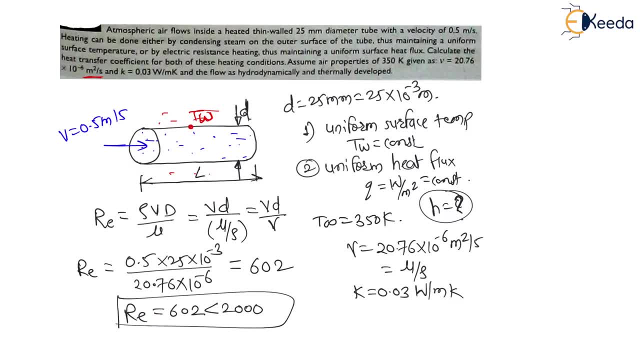 for flow through pipe when your renal number is less than 2000, it is called laminar flow. this is called laminar flow, right, therefore, here the flow is laminar. now first, for laminar with constant surface temperature, we have to calculate convective heat transfer coefficient h and second, 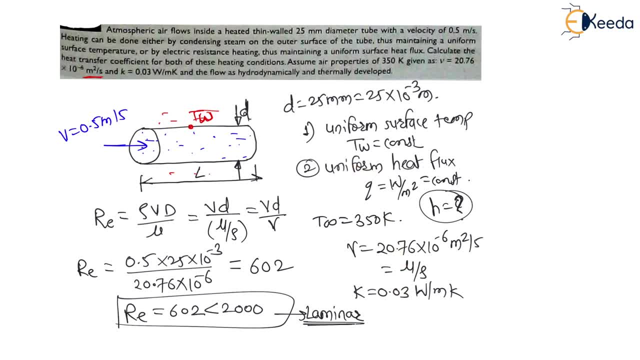 for laminar with uniform heat flux we have to calculate convective heat transfer coefficient h. so let us solve this question now. very first is for laminar: for laminar and fully develop- here they have mentioned hypothalamically and thermally developed. for laminar, fully developed with constant wall temperature, with constant constant wall temperature. 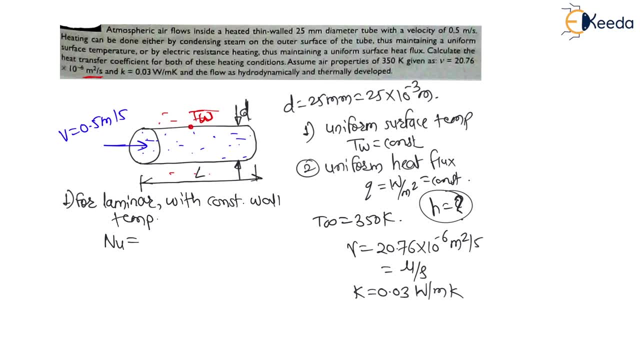 for this condition, the nasal number is constant and the value of nasal number- this value, you must remember, very, very important for competitive exams- or laminar, or laminar flow through pipe, for fully developed, developed flow with constant wall temperature, the nusselt number is 3.66 and this nusselt number is: 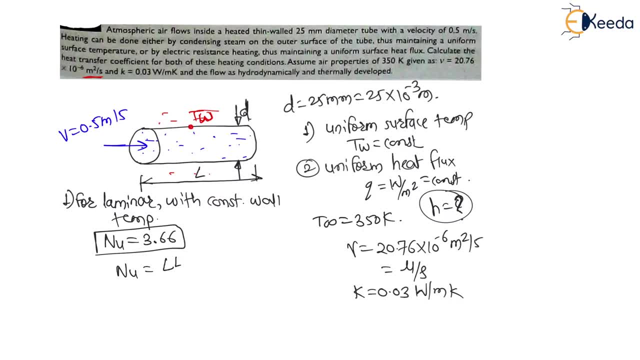 nothing but nusselt number is h? l. here the formula is h? l divided by k, h? l divided by k, where this l is diameter. right, l is characteristic dimension and for flow through pipe it is a diameter. therefore, instead of l, i will write here diameter, otherwise you will get confused. right, it is hd. 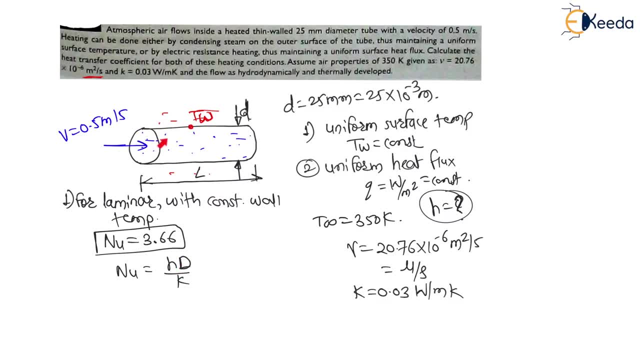 divided by k, these characteristic dimension and for flow through pipe, the characteristic dimension is diameter, right, therefore, here, this nusselt number is 3.66, is equal to eh into diameter, is 25, into 10, to the power minus 3, our thermal conductivity is 0.03 right now in this equation.